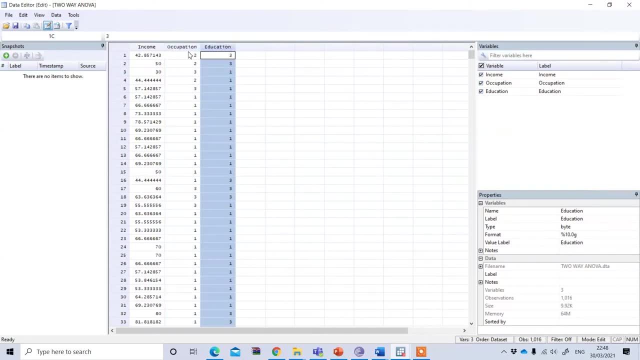 actually two independent variables and both are categorical and each of this independent variable has several group. so basically, occupation has three group and uh, for example, um, two means the government jobs, three could be business, one could be private job, same the education. it has decoded as a uh, total three groups. so three, one and there is an option for two as well. uh, now for this. 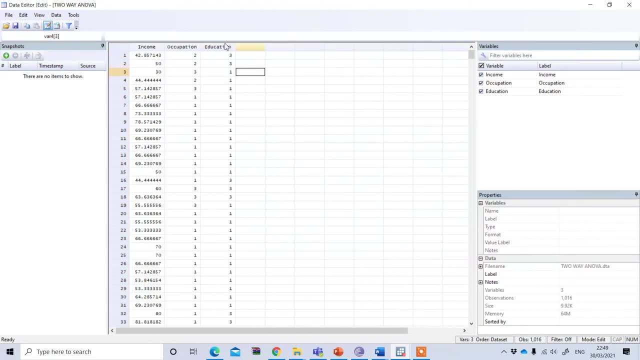 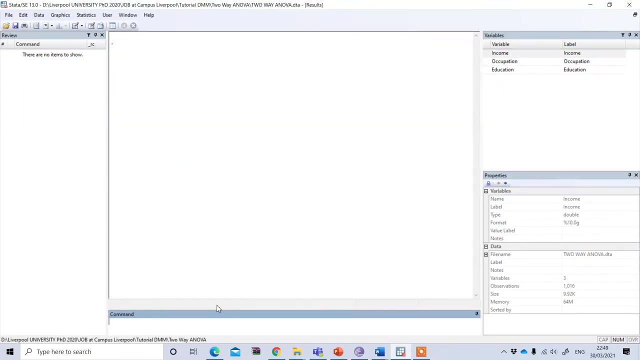 education. this these three groups actually indicated by example. one means um school, uh two means college and three means university. okay, let's perform this to a anovines data. to do this, i have to type the command anova and then my dependent variable, which is actually income. 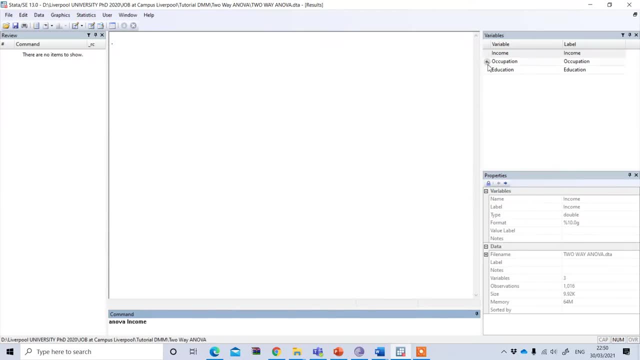 and then i have to put one independent variable- occupation, and to slash, and then our another independent variable. okay, so you see anova dependent variable and two independent variable in between, two slash, and then if you press enter, it will too, you will get the result of the two-way anova. 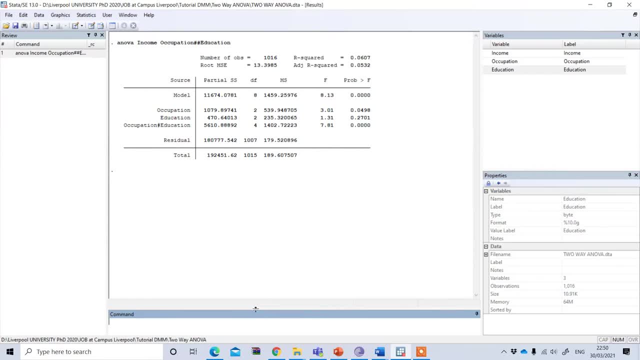 now from this table. you can interpret like um if you see the p value and this is the interaction, right, the interaction, the joint effect of occupation and education, and it is statistically significant. This is also statistically significant at 5% level, but education is not statistically significant. 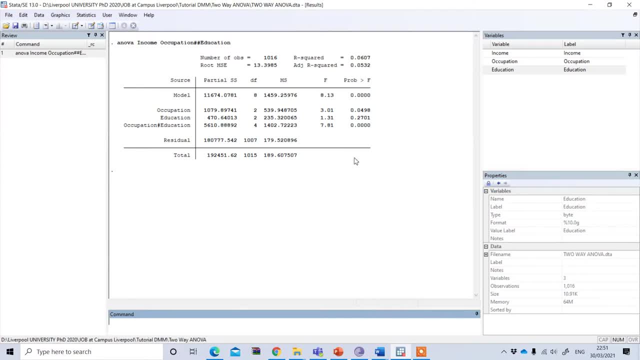 That means, if I want to explain this table, this means income. this actually significantly varies according to different groups of occupation, Because it is statistically significant. However, the income, it doesn't significantly differ according to the education category for our sample data, because it is not significant. 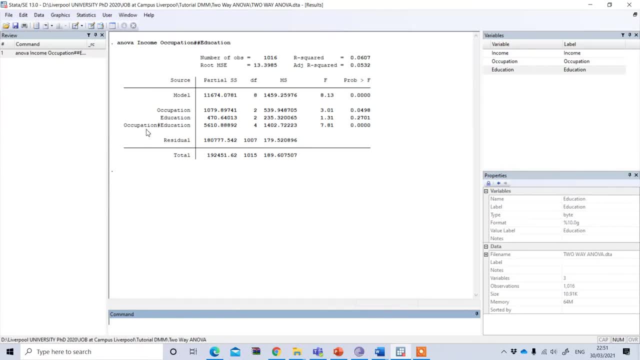 However, occupation and education, these two variables can jointly affect our dependent variable And it is statistically significant. You see, it is less than 1% or even less than 0.01%. Now, if you want to see the mean difference, we can perform the post-hoc analysis. 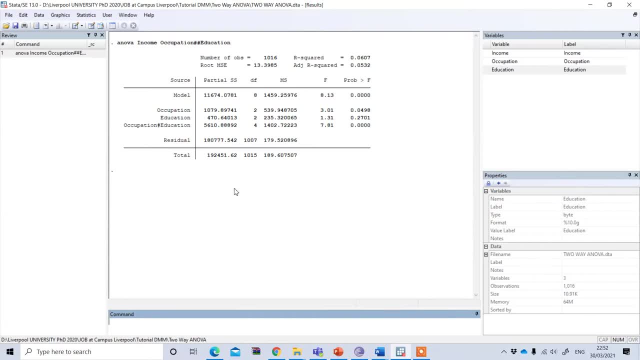 So to perform the post-hoc analysis we can use Bonferroni-Tacchi and some other method. So for this example, let's see how these different groups of the occupation actually differ Because education it says that non-significant. so we don't need to actually see the difference between the mean effect of the different groups under the education because it is not non-significant. 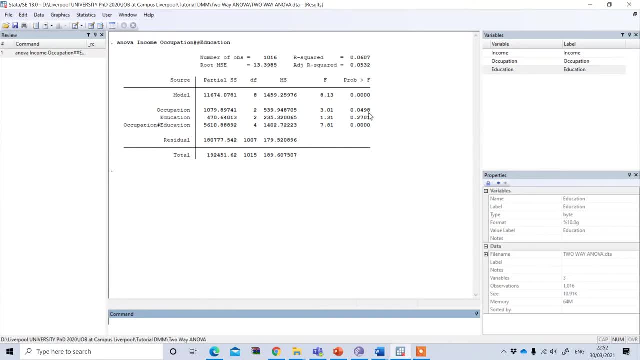 However, since the occupation, this is statistically significant, then we can see which group actually significantly differ than the other groups in terms of the income. So to do this I can write: I can write pw, mean, and then our dependent variable, which is actually income, and then comma over the variable that is the independent variable. 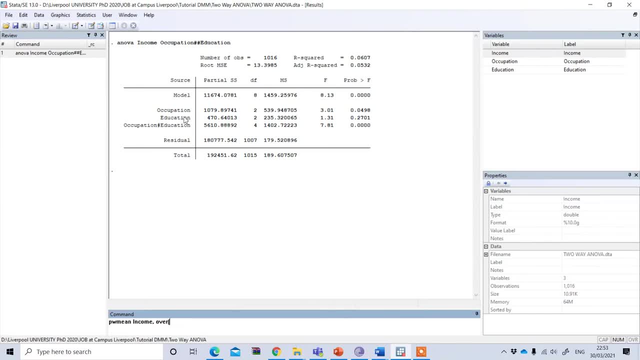 And we can perform in terms of education. but what I said earlier, it is not necessary because it is non-significant. so I will actually use this occupation, the significant one, So I put this significant independent variable And then, after the bracket, I can write m compare. 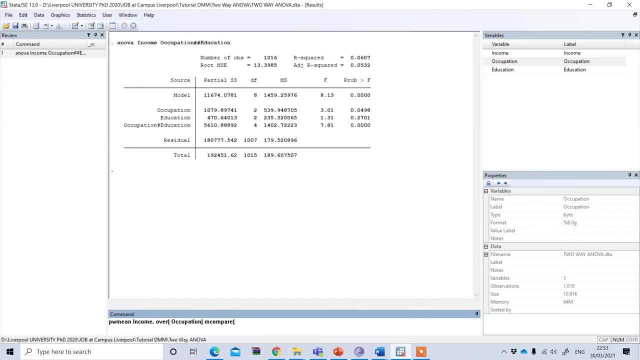 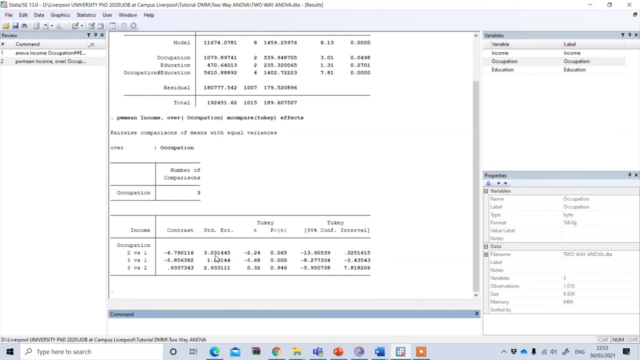 And then the relevant test. you can use the Bonferroni-Sedac, I am using here Tacchi, Okay, And then effects. And if you, If you, If you press enter, you can see the mean differences. 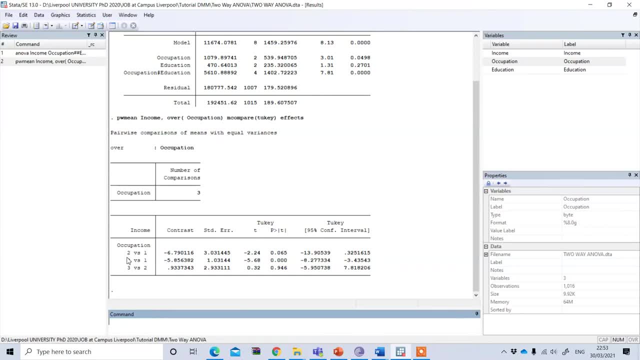 So especially you see 2 versus 1, and this contrast is minus 6.. This mean the mean income of occupation group 2, it has 6,000 pounds lower than the group 1. And it is- And it is not statistically significant at 5% level, but if you consider the 10% level, but then you can say that it is statistically significant at 10% level but not at 5% level. 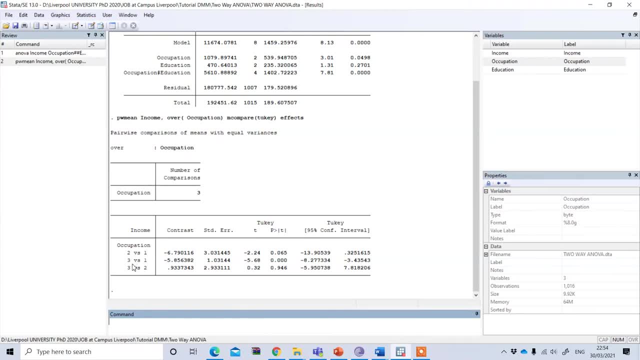 However, if you see the 3 versus 1,, this means that occupation. So, for example, 3,. if 3 is the private job, then you can say the private job holders has lower income than the group 1.. So, for example, if 3 is the private job, then you can say the private job holders has lower income than the group 1.. 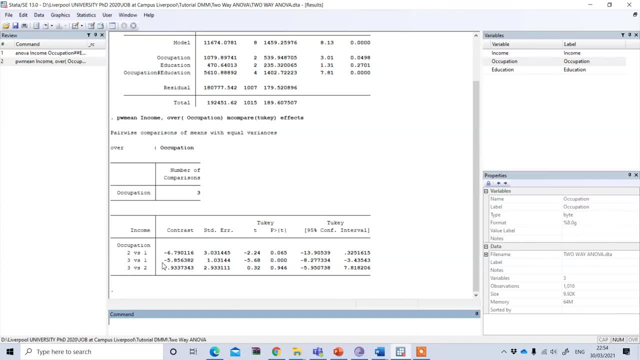 That is business group And this is actually difference. Here is actually 5,000 pounds And this is statistically significant, Right? However, compared Comparison between 3 and 2, and it is actually non-significant. So in this way you can also find the- you know, the mean difference under the post hoc analysis. 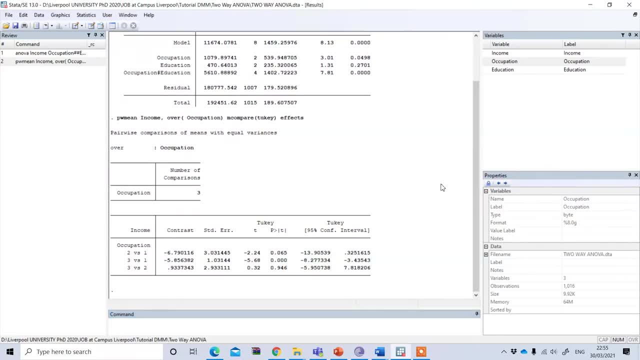 So in this way we can perform 2A ANOVA in the startup. Thank you. Hello and welcome to the Cybrary IT secure coding course. My name is Sunny Ware and we will be going on this journey together, learning about secure coding techniques, as well as how the attacks are done and the appropriate mitigations and countermeasures that we can put into our application. 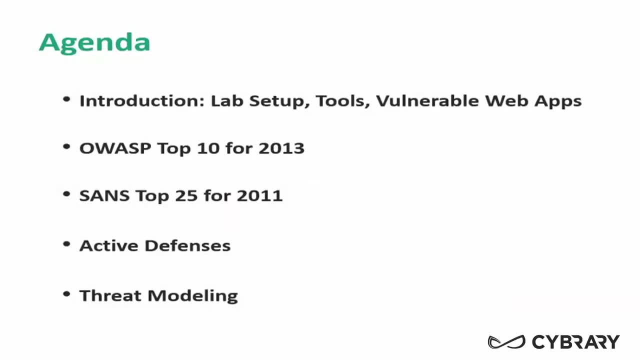 code. So our agenda for this course is: first there'll be this introduction, which is what you're watching now. We're going to have some additional videos that go through the lab setup, some demonstration about some tools that we're going to use, and then a very short description of the